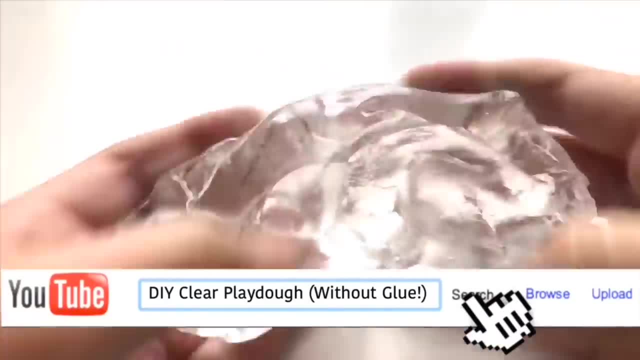 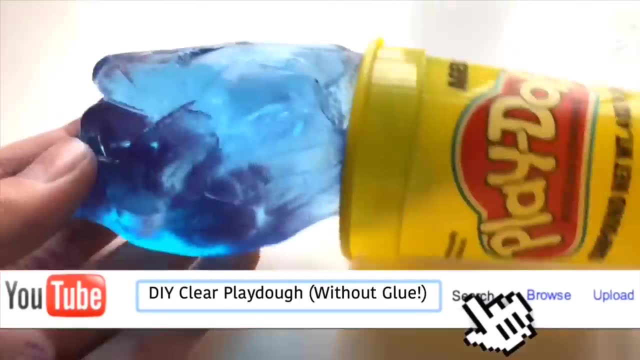 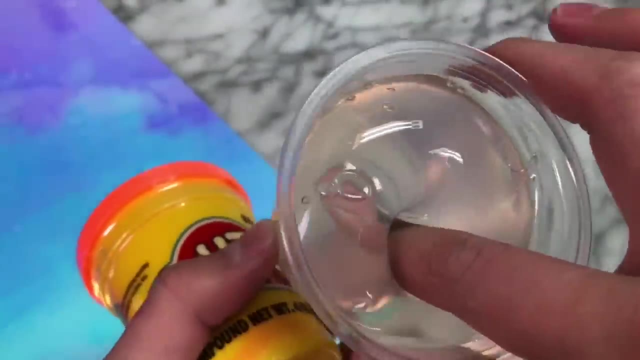 Hey guys, it's JaceHGY and welcome back to That Beciding YouTube. Today I'm going to be showing you guys 10 different ways to make clear play-doh, and without any glue. So don't forget to stick around to the very end of this video to learn how to make clear play-doh with ingredients you. 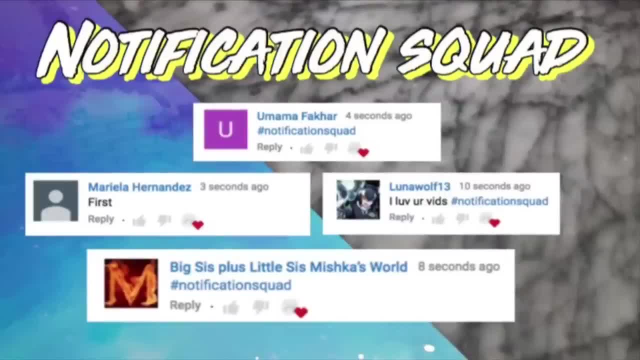 already have laying around your house. The notification squad shoutouts of today's video go to Anamafikar Le Hernandez, Lunable13, and Big Sis and Little Sis Mishka's World. So if you would like a notification squad shoutout and get to be in my next video, all you have to do is be. 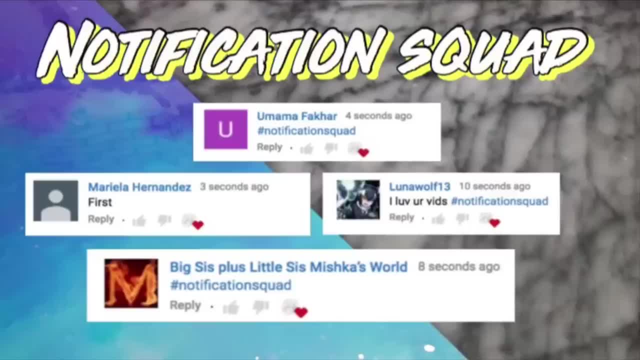 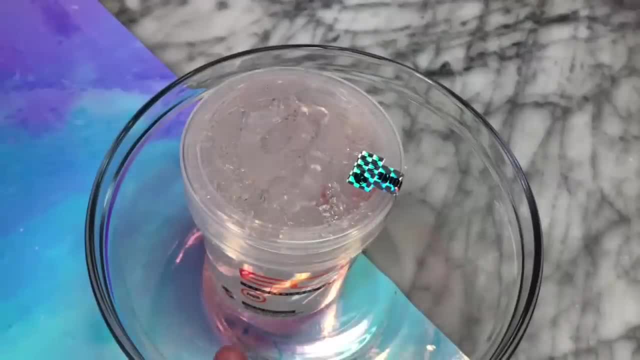 subscribed, have the notification bell clicked and comment down below notification squad when I post my video, and I will do my best to give you one in my next video. The first clear play-doh recipe I'm going to be testing out is clear play-doh made from hair gel To make this recipe. 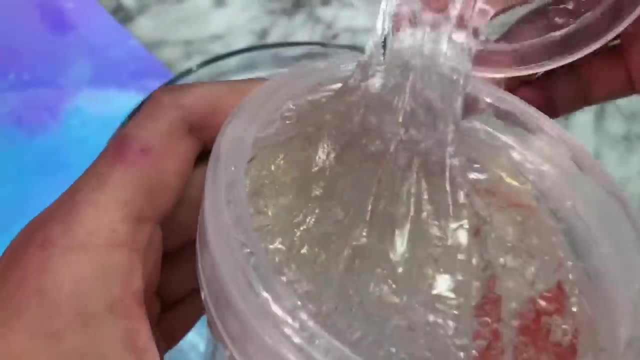 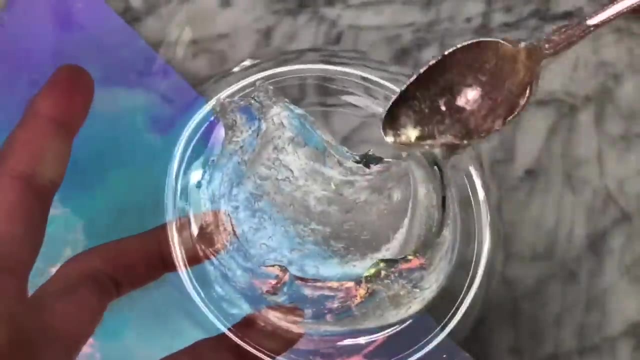 you're going to be needing some alcohol-free hair gel Now. it is very, very important that it is alcohol-free, because if you microwave hair gel that contains alcohol, it will blow up in your microwave. But to make this recipe, you're going to be needing a spoonful of. 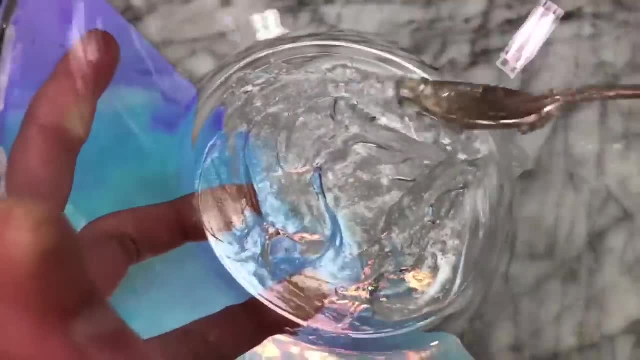 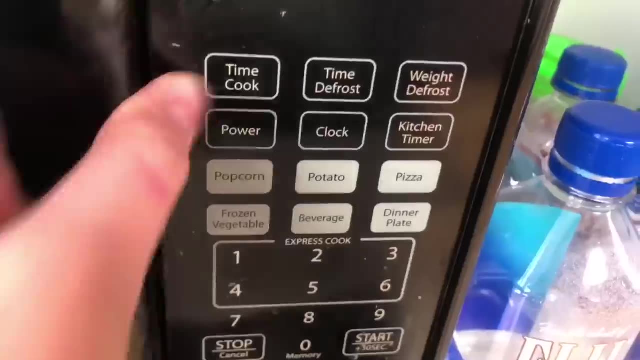 that alcohol-free hair gel and you just want to put it in a microwave safe bowl and spread it thinly on the bowl so that the hair gel will dry out and create clear play-doh. Once you have done that, all you have to do is microwave it for 30 seconds and then we're going to let it cool off. 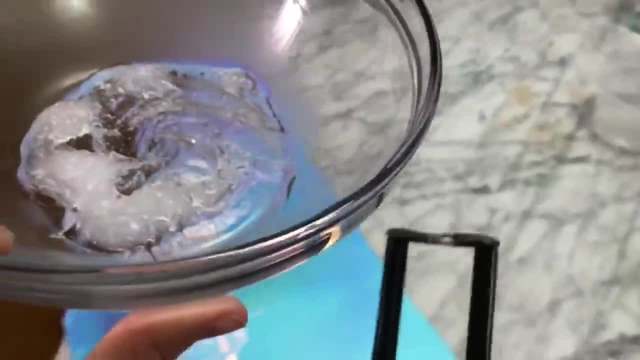 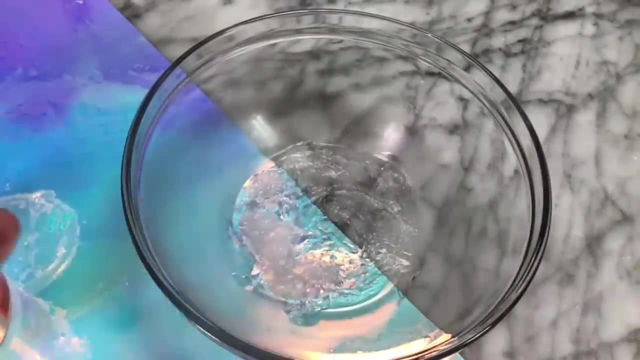 before we check to see if it actually did turn out to make clear play-doh. I just pulled this out of the microwave and I do see that some sort of a reaction happened because the hair gel in certain places is a little bit murky, but I'm going to let this cool off. 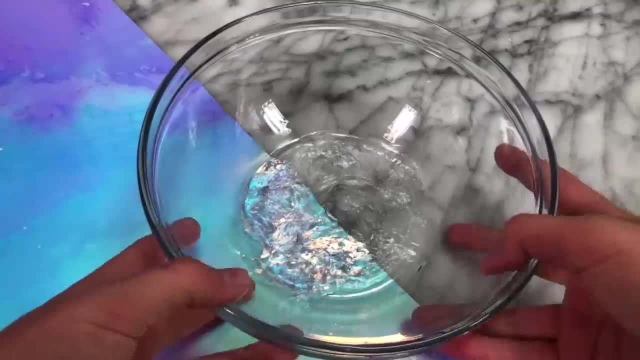 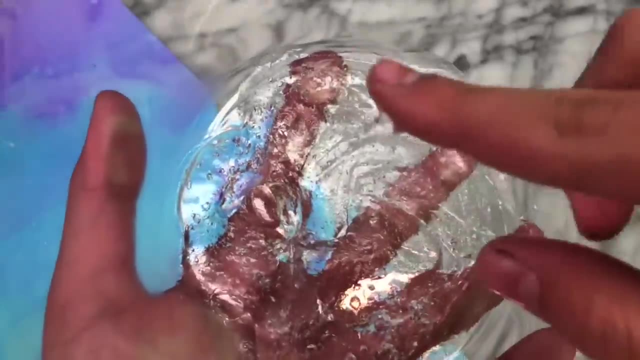 For about a minute or so, and then we're going to check on this and see how it turned out. The hair gel has cooled off for about a minute, you guys, so I'm going to feel it now. I'm super excited. I don't think it has turned out, but we'll see. Okay, guys, I'm feeling it right now and, as you, 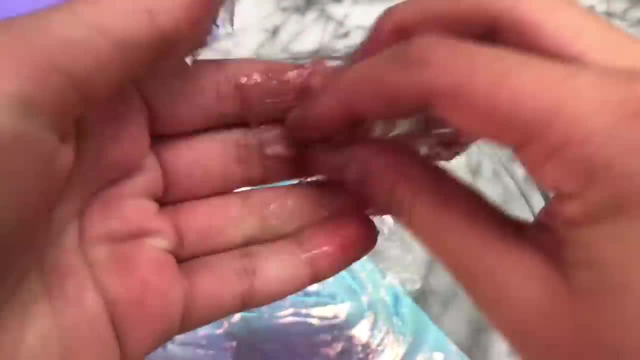 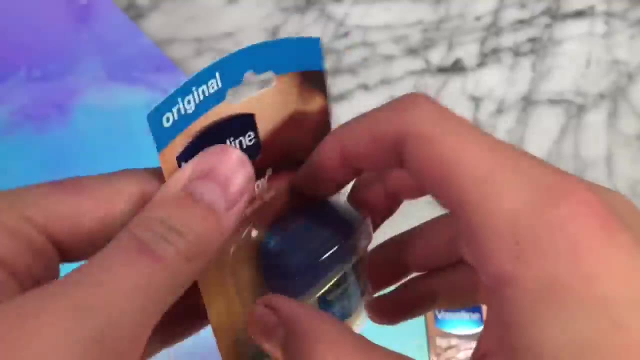 guys can see, it's super sticky and did not turn into clear play-doh. so I'm pretty sure, unfortunately, this recipe was a fail. but let's test another one and see if we have more luck with the new method to make clear play-doh out of Vaseline. So I'm going to be testing two ways to do this, so I 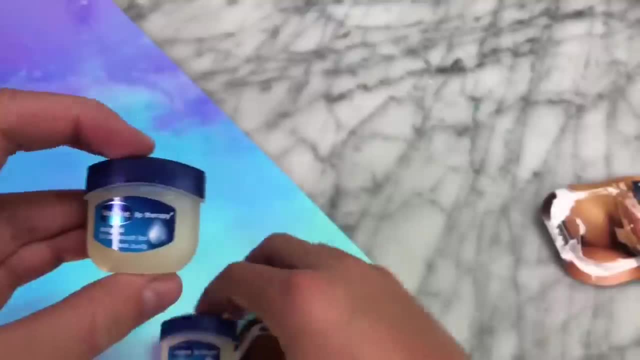 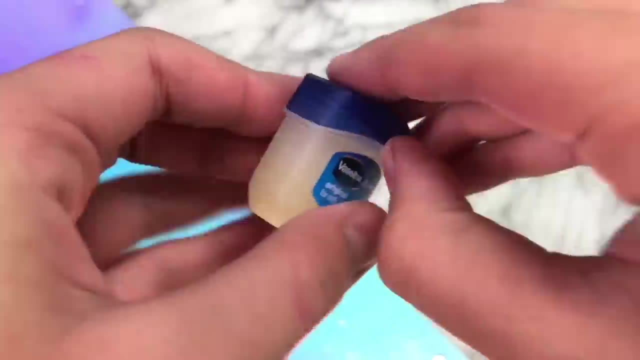 got two little Vaselines. I'm not sure why, but I really think everything is so cute when it's tiny. so I got the little tiny Vaselines, but I have two containers right here so I can test both of the recipes and we'll see what happens. The first Vaseline, clear play-doh, we're going to be testing. 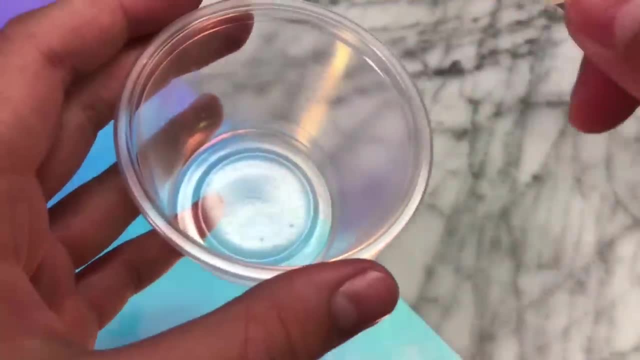 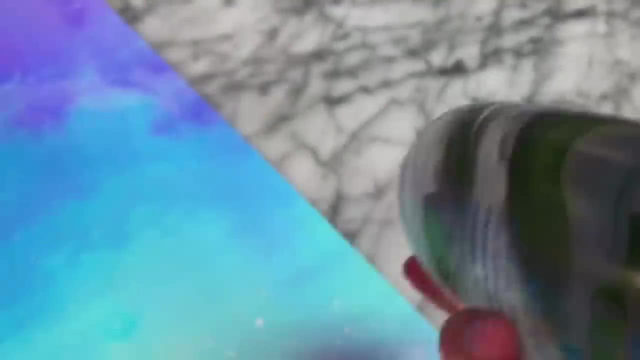 out is mixing Vaseline in thick clear shampoo. Once we mix those two ingredients together, it should turn into clear play-doh once refrigerated. so I'm going to take a good scoop of that Vaseline. Basically, when you're making clear play-doh, your goal is just to make 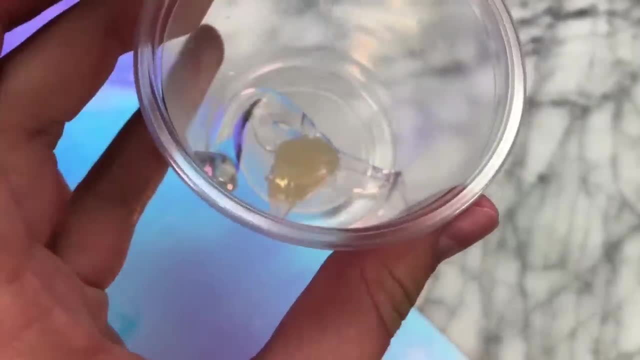 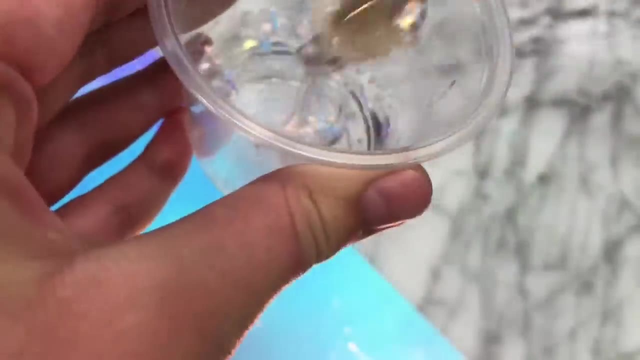 the thickest slime you can possibly make and then let it dry out. For this recipe, you'll need a thick clear shampoo. I'm using the OGX one. As you guys know, this is my favorite clear shampoo to make no glue slimes with, so I just mixed some of that in, and because I added 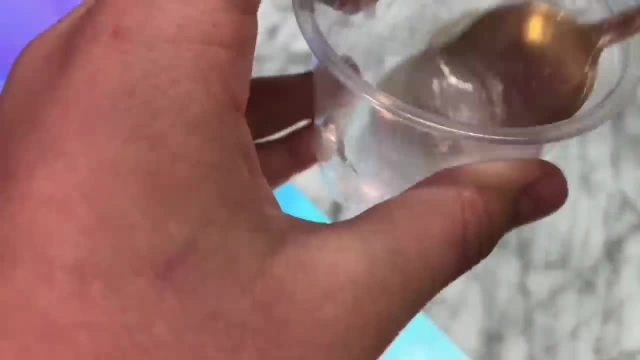 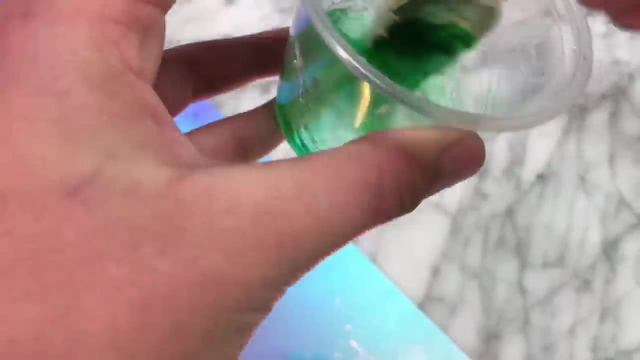 a lot of Vaseline. when I mixed it it stopped being clear. so this was my first sign that this recipe probably wasn't the best one. To make it look a little cooler, I added some green food coloring. then I had to refrigerate it because it was not really turning into slime or even anything close. 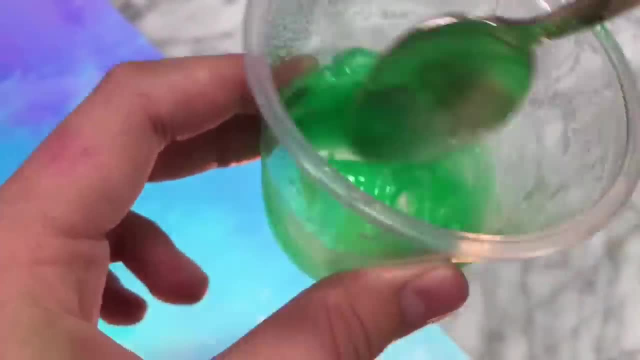 to a clear play-doh, so I refrigerated it and then I added some more Vaseline. So I'm going to mix it up and this is how it turned out. As you guys can see, it formed a little bit of ice crystals, except for not enough to make it thicken up, so when I mixed it it just started melting a little. 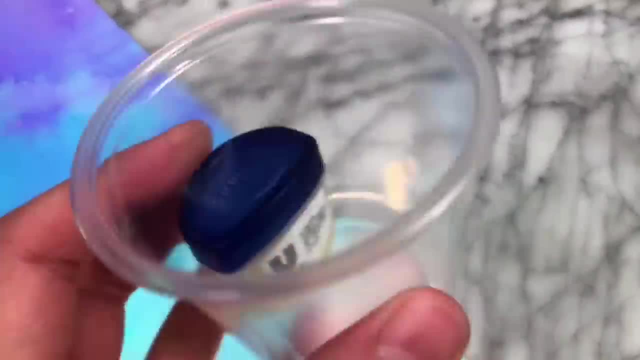 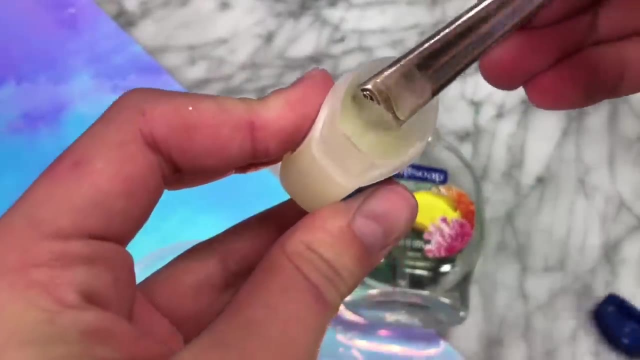 bit more and made this big gooey mess. This was a huge fail, but for this next one, we're going to be testing mixing soft soap and Vaseline. For this, I'm going to be adding a lot less Vaseline. If this recipe does work, I want it to be a little more clear than the last one, because the Vaseline 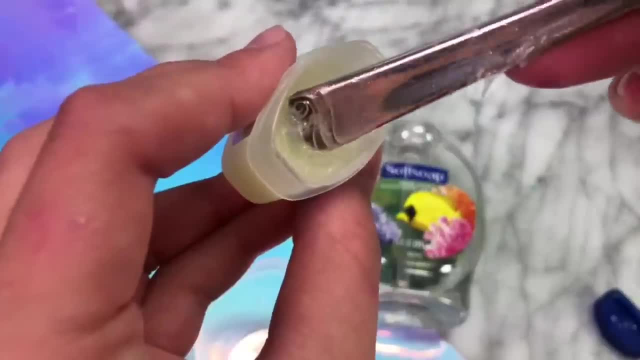 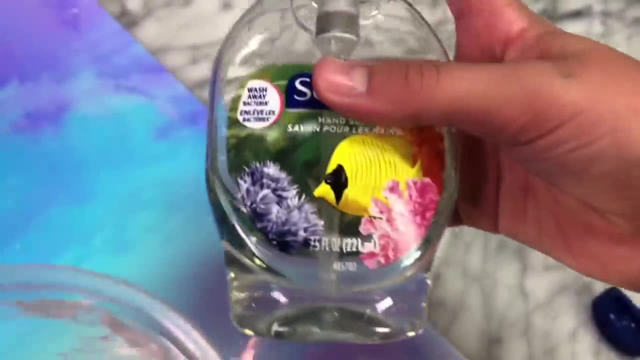 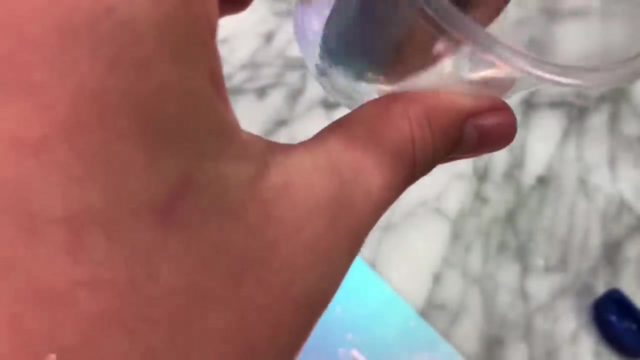 basically turned the shampoo into a white shampoo, which wasn't ideal for making clear play-doh, because the whole point of it is, it, is clear. So I added some Vaseline and then I finally added my hand soap. For this you can use any hand soap, because hand soap, I have found, doesn't vary as much in texture, so just use any hand soap. 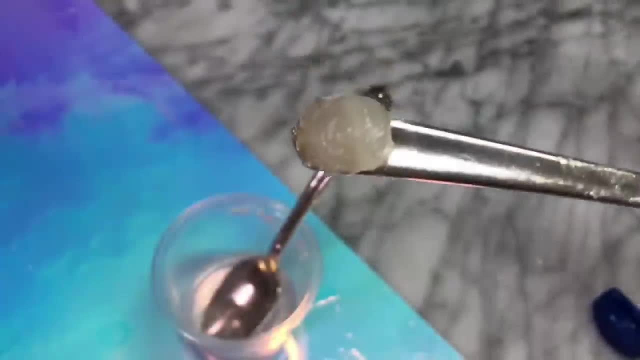 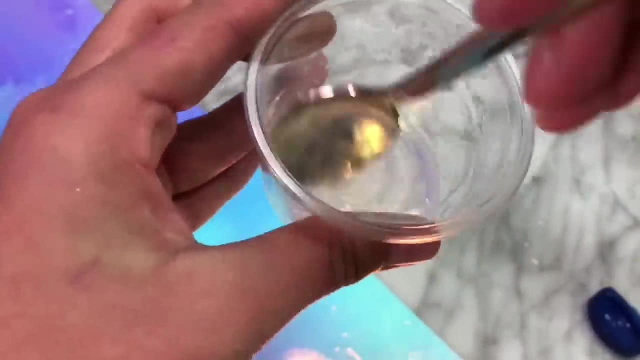 for this. I did add a little bit more Vaseline because I feel like that amount of Vaseline I added wouldn't really do anything. so I added that in and I gave everything a good stir, Mix it super, super well. This helps a lot when you're making soap slimes and then you are going. 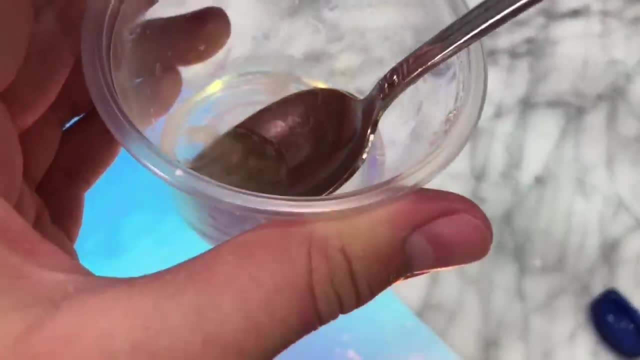 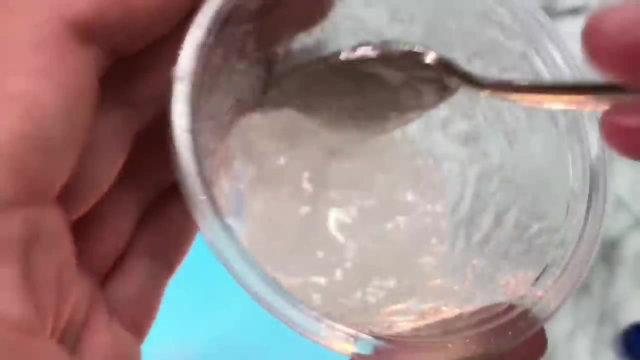 to need the cream of tartar If you guys don't know this already. cream of tartar is like the key factor of making normal play-doh, So I thought this one would probably work, but I kept mixing it and it really was a fail. I have 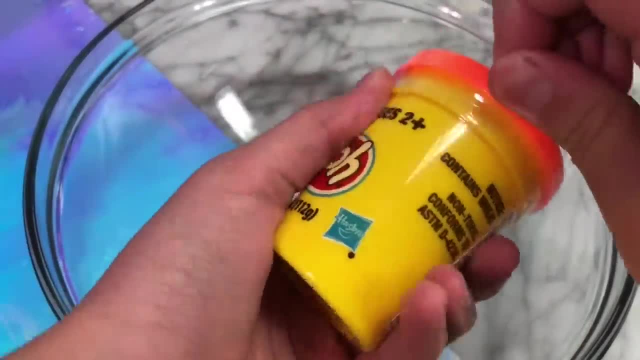 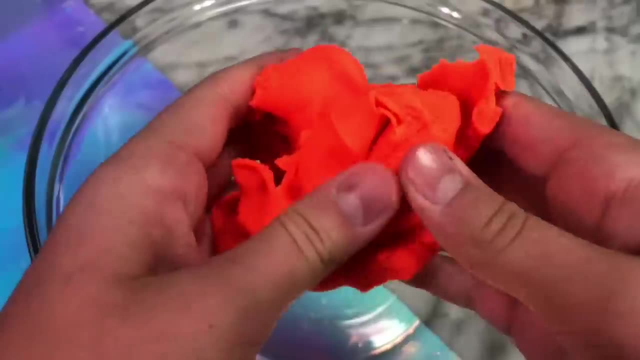 high hopes for this next clear play-doh recipe, because we're actually going to be using real play-doh, so for this one you're going to be needing real play-doh. This is a great way to make clear play-doh if you don't have cream of tartar. I do have to say I have tested this recipe before. 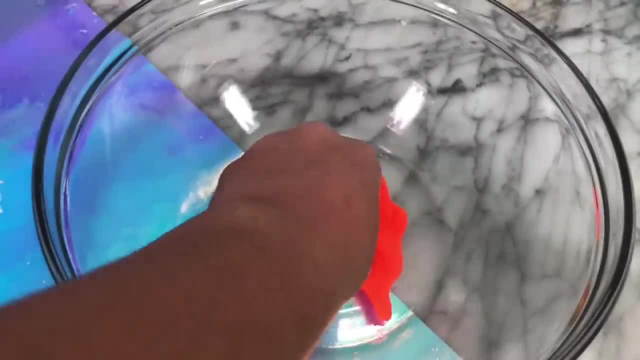 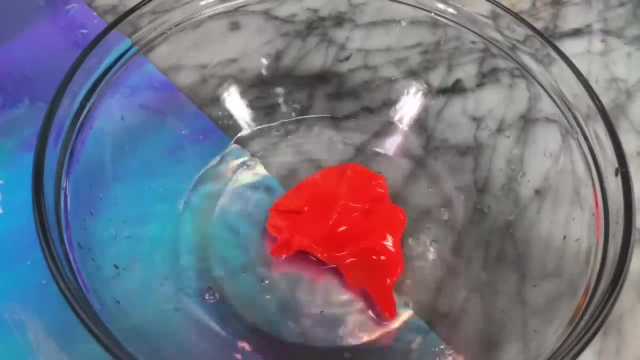 so I do know how it turns out. I won't tell you how it turns out yet, but I have changed a couple of the ingredients so that it will work super great today. but I'm going to just add some water into the play-doh so that it will soak. 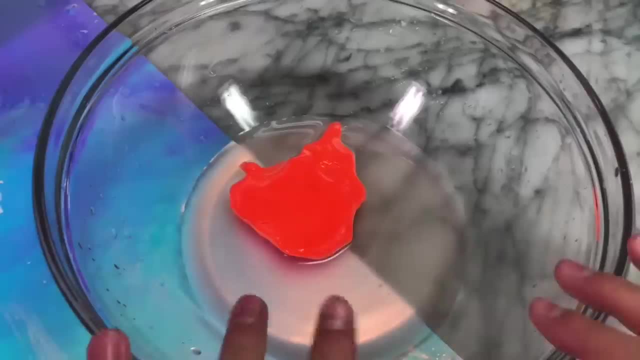 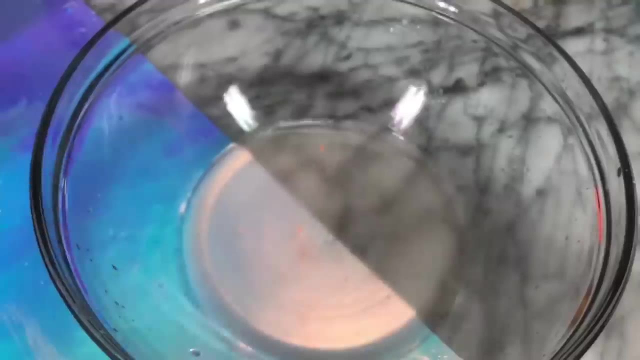 This actually wasn't Evian water. I just had this empty Evian container and I needed to put some water in here, so I just decided to use it so I could store the water in it. But once you have let it soak, you just want to take the play-doh out and you will have your cream of tartar water. 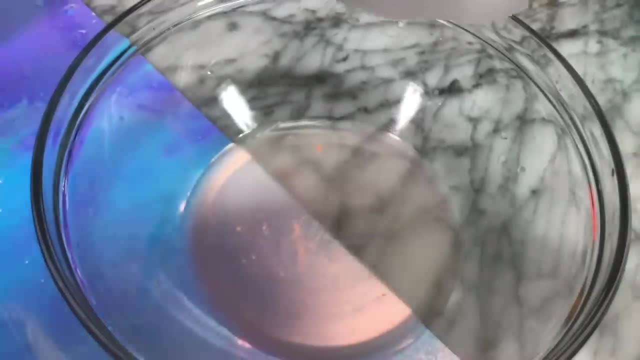 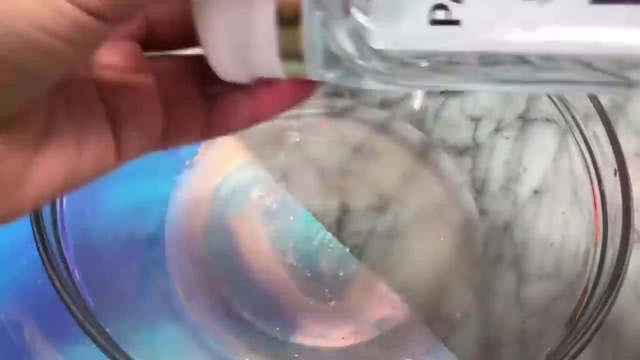 For this you're going to be also needing some thick shampoo. You could use white shampoo for this also. I have tested it with white shampoo, but it won't give you a clear play-doh, so I guess that kind of defeats the purpose of making clear play-doh. but once you have added the shampoo, 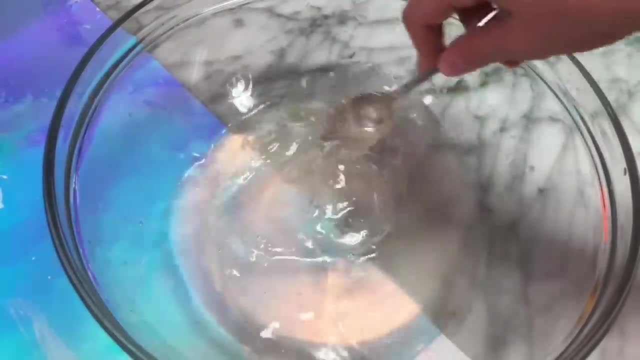 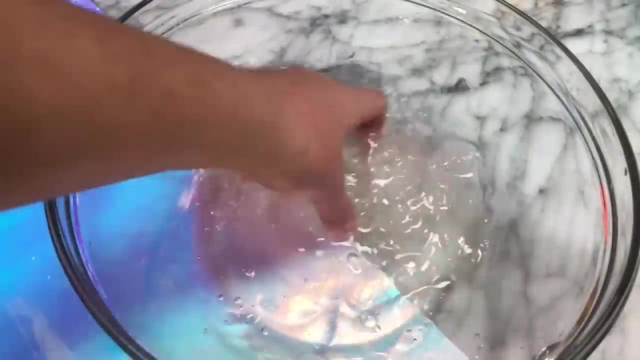 in the water. I'd recommend adding cream of tartar in there too, just because the cream of tartar that actually comes out from the play-doh once it's soaked is very little, so you can get by by using that, if you let the play-doh 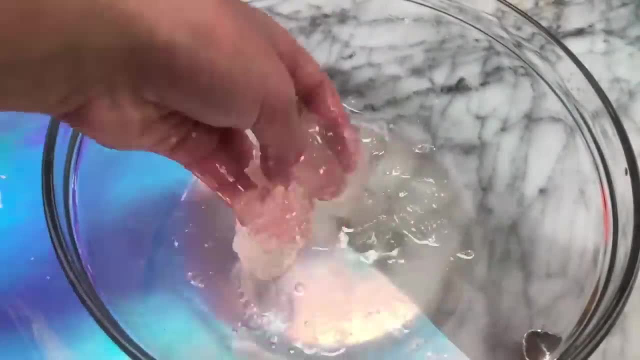 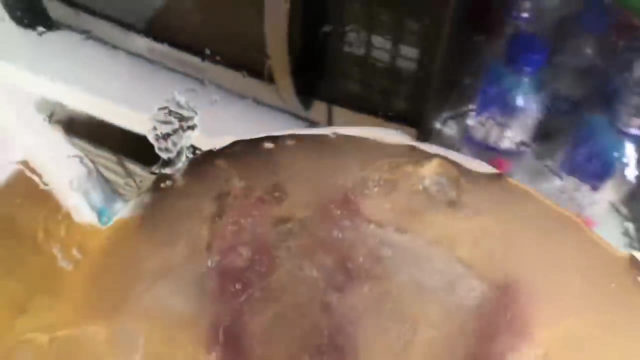 sit for a long time and soak in the water. but I just added some more cream of tartar because I didn't let it soak for very long. but once I mixed it it turned into kind of like a clear slime, except for it wasn't moldable yet, so I microwaved it so some of the water would evaporate out and 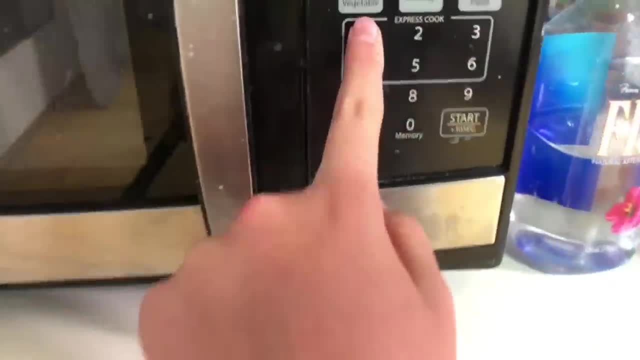 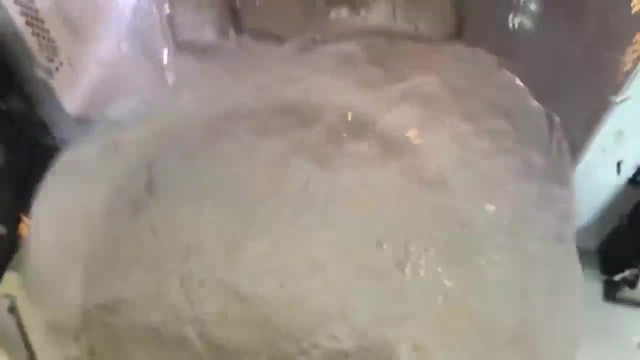 we would end up with a clear play-doh, hopefully, And I will be microwaving it for one minute, but just check in with it to make sure that it is good. My microwave is very dirty, by the way, because I use this microwave strictly for slime, but once you have taken that out, you want to feel it. 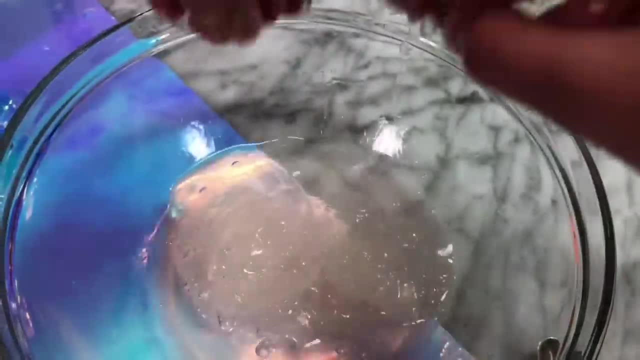 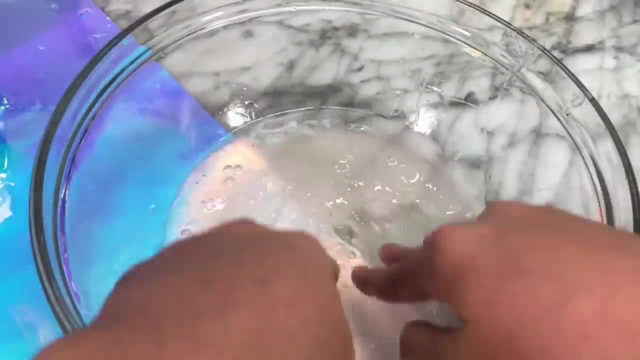 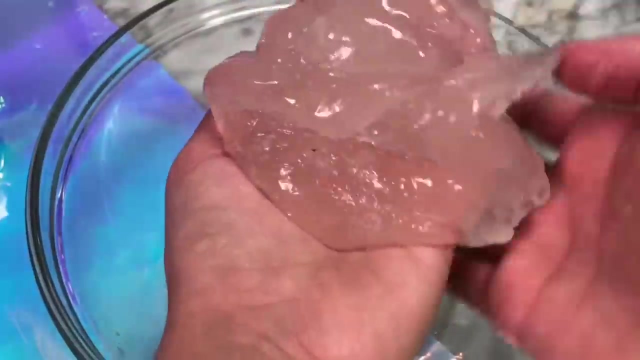 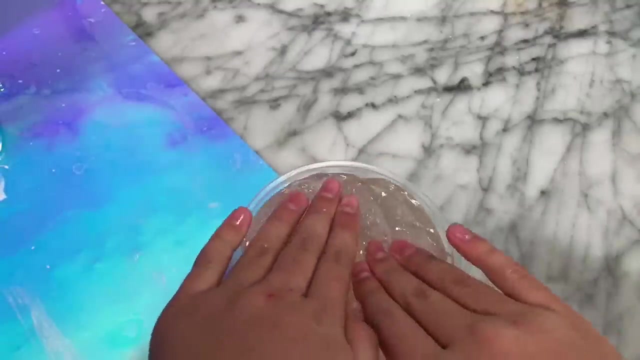 it should make a pretty good slime. Now it is going to be kind of melty from the microwave, so just play with it until it starts drying up a little bit, And then you can store it in an airtight container and it will get harder over time, which will give 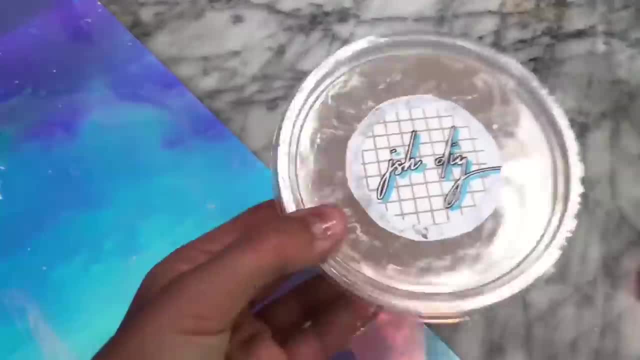 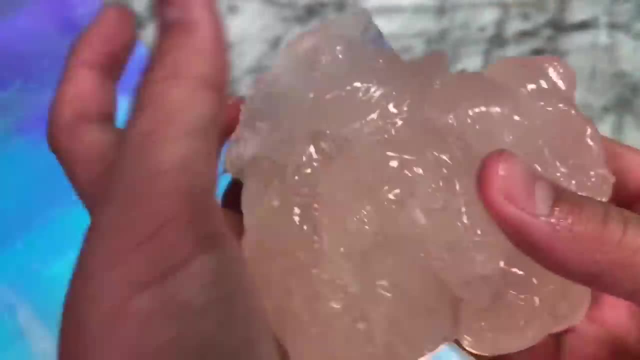 you more of a clear play-doh texture, so just store it in there. If you're wondering why this is different from slime, it is different because it is moldable and once you mold it it should stick and stay in that shape for a little bit longer than normal slime would. For the second to last, 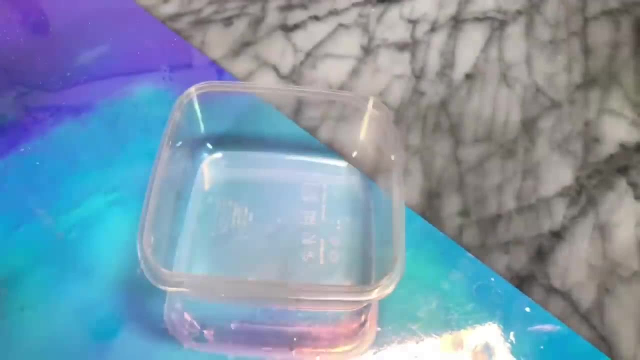 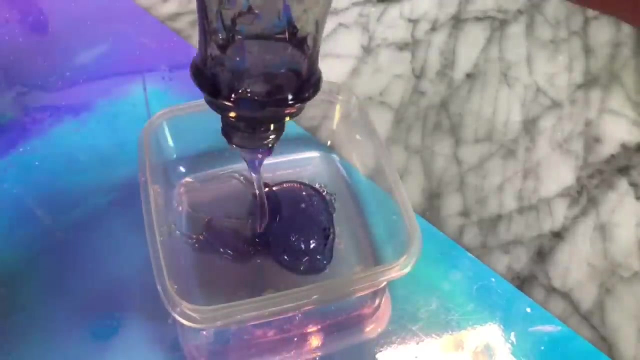 clear play-doh slime recipe we're going to be testing. I'm going to be testing dish soap shampoo- clear play-doh slime. Now, this is not really a recipe because I did come up with it myself, but, as probably know, dish soap shampoo slime is a great slime to make if you have no glue and want to make. 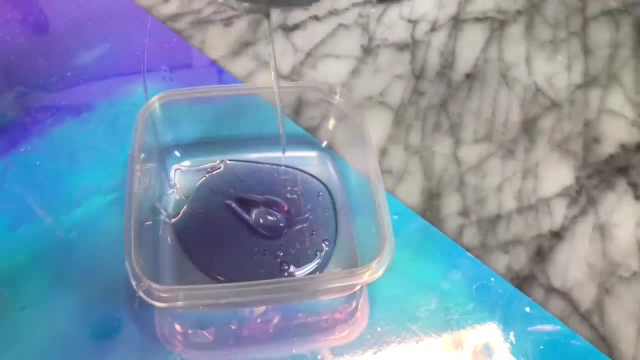 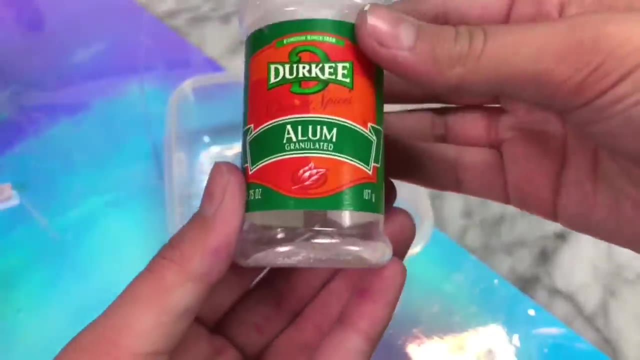 a thick, clear slime. so I thought, if we made a dish soap clear slime and we let it sit out for a little bit, that it might turn out kind of like a clear play-doh. If you would like to recreate this recipe right now with me, all you're going to need to do is combine even amounts of dish soap and 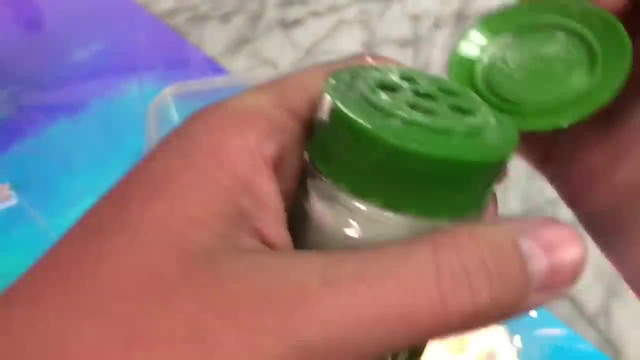 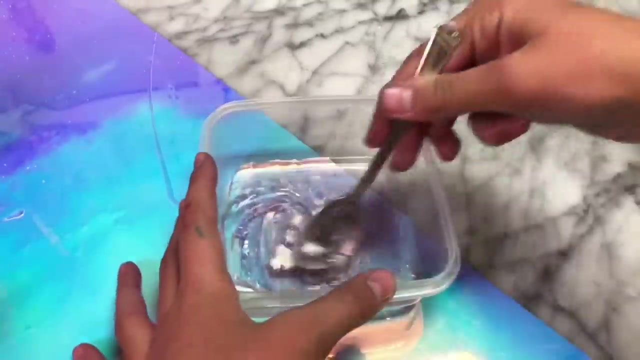 shampoo in a container and then add some cream of tartar and alum into it. and, by the way, do not forget the cream of tartar, because this whole recipe should be dependent on it. if I end up doing this and it works out correctly, Because the cream of tartar will give you that putty or clear play-doh like texture or consistency. 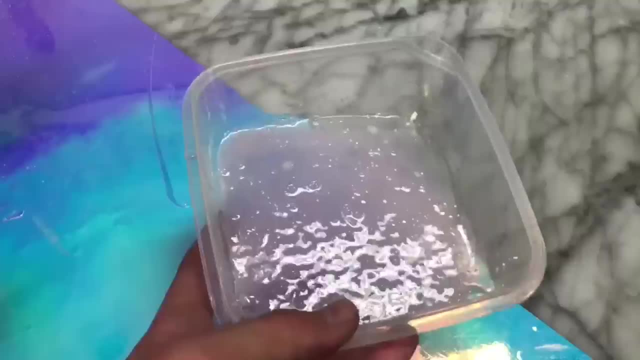 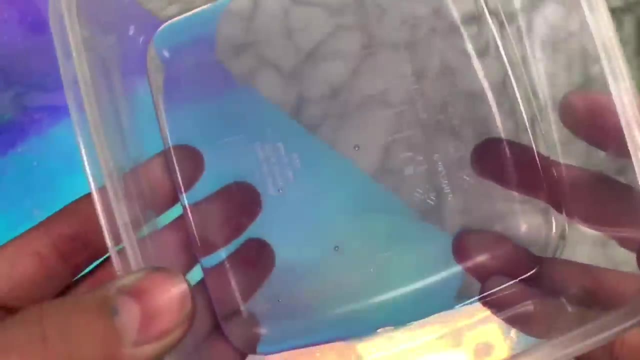 and also don't forget to mix it a lot, because the cream of tartar does activate by mixing. So once you have all those ingredients in your bowl and you've mixed it all up, let it sit for a couple of hours and you should have a nice crystal clear mixture of what I thought was going to be. 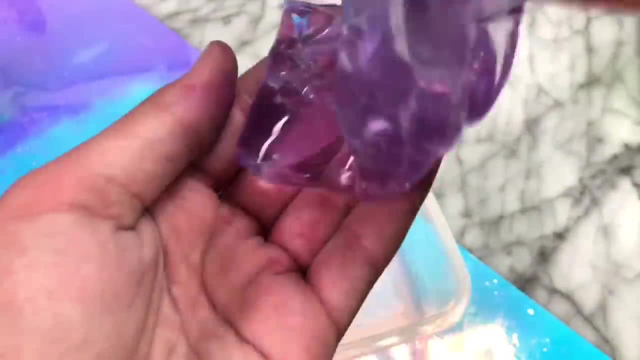 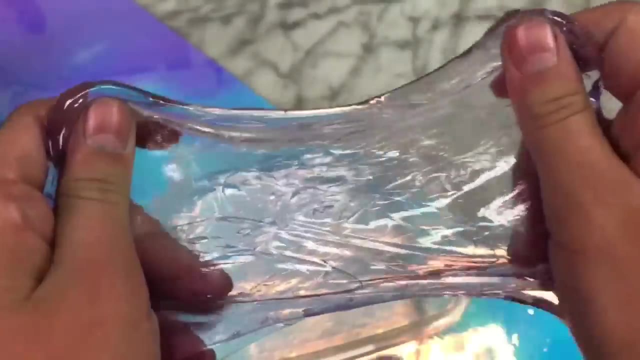 clear play-doh. but once I started poking it and then took it out, I soon realized was basically just a normal no glue clear slime. I would probably say this was a fail, but then again it did make some pretty good slime. so if you're looking to make a clear slime, I guess it works for that. but I 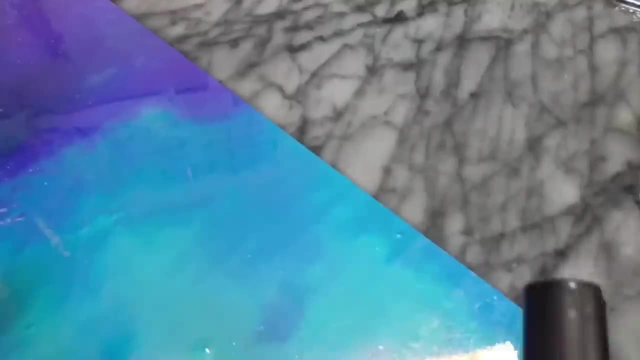 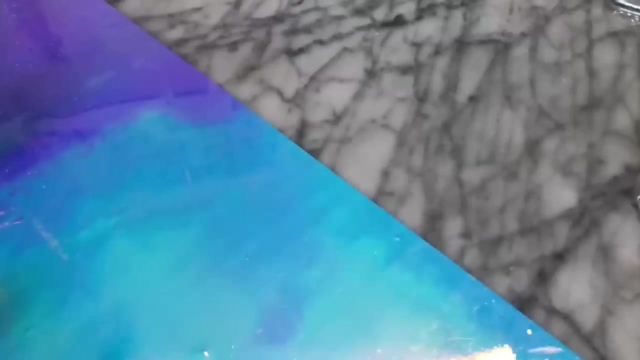 would definitely not call this a clear play-doh because it was a little too stretchy and kind of sticky. Final clear play-doh recipe I'm going to be testing is the original clear play-doh recipe, so I have high hopes for this one, because I have heard some good reviews by you guys of this recipe. 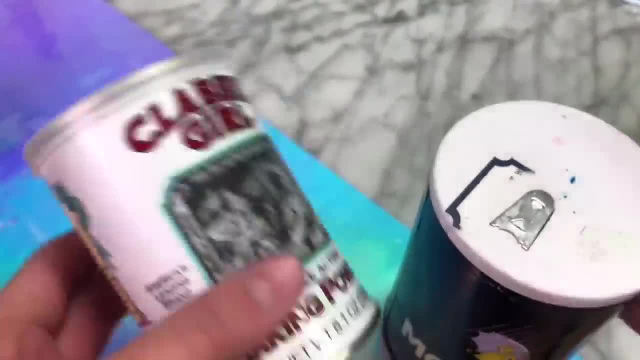 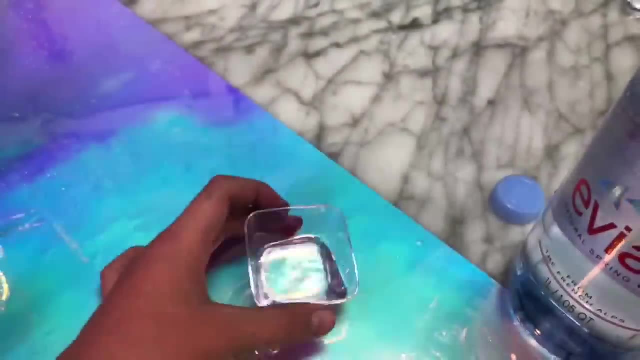 working. So for this you're going to be needing some anti-residue shampoo, some cream of tartar, or you could use baking soda or salt and some water. So to start this recipe off, you need to take a container and add some water into it, and then you have to add some cream of tartar. 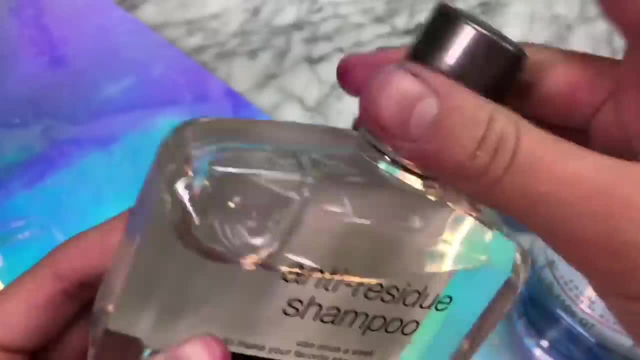 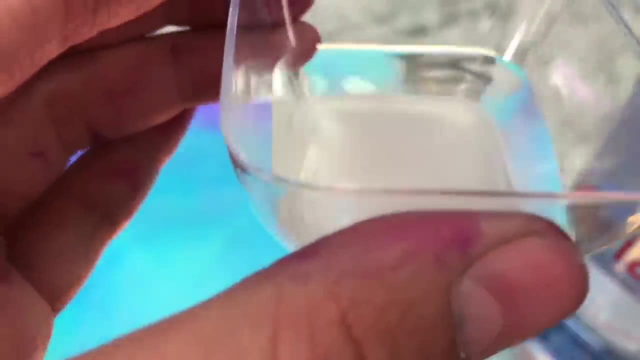 But you apparently can use the salt and baking soda, but when I tried that earlier today it didn't work, so I would not recommend doing that. Once you have made your clear play-doh activator, which is the cream of tartar water, you're going to need to add some of your anti-residue shampoo. All the